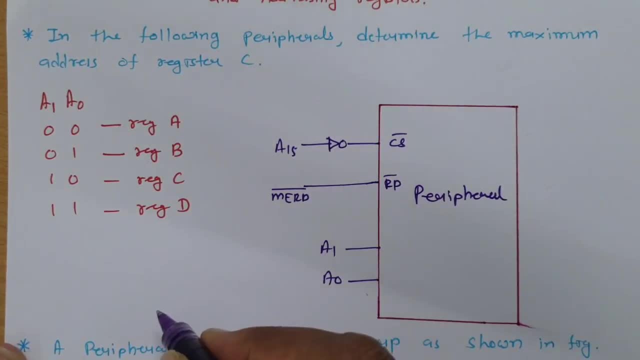 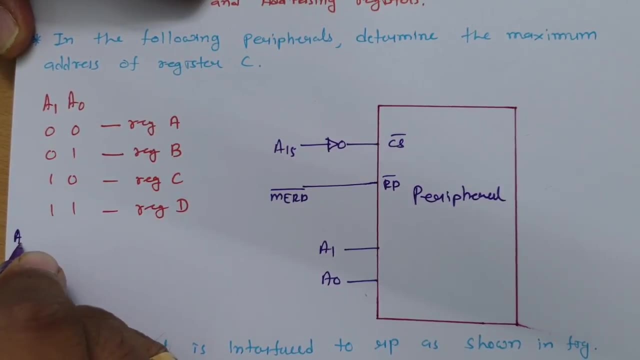 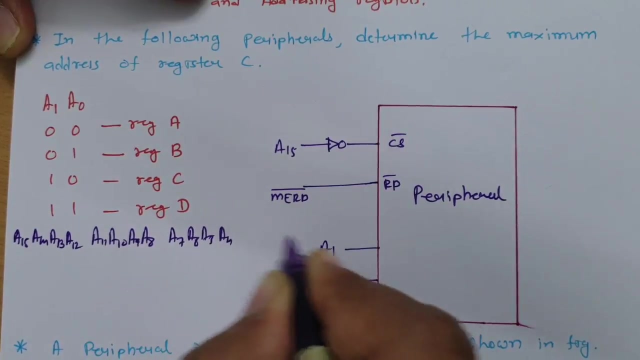 So for that we need to write all possible addresses. So here I will be mentioning that, all possible addresses, So starting from A0 to A15.. So here I have A15, A14, A13, A12, 11, 10, 9, 8, A7, A6, A5, A4, A3, A2, A1 and A0. 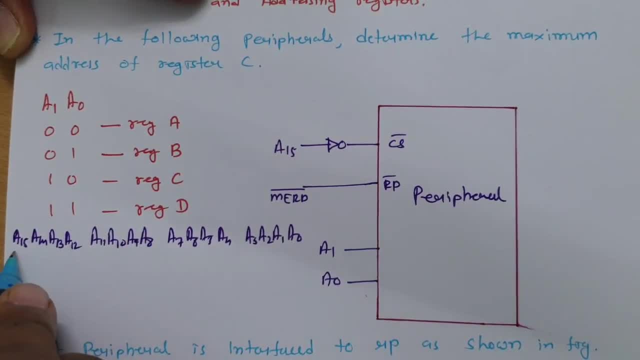 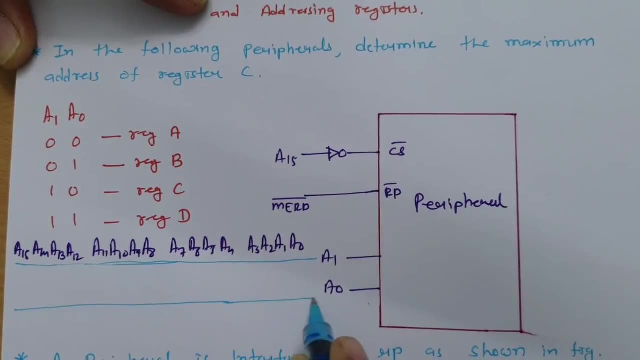 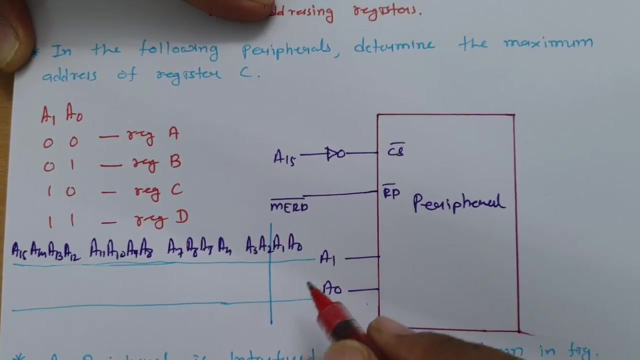 That is how addresses are there, And now in this address we have resistor C selection, right. So resistor C selection, resistor C selection: that will be getting done by A0 and A1.. So resistor selection: that will be getting done by this. And for: 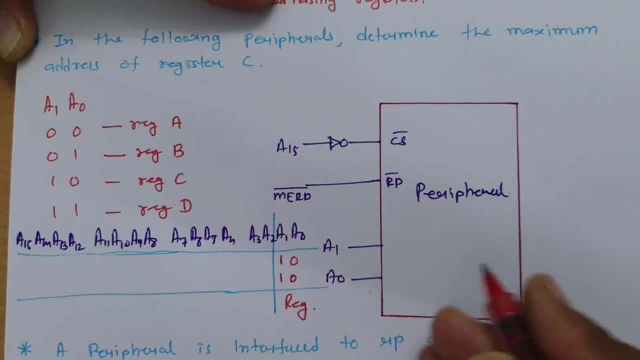 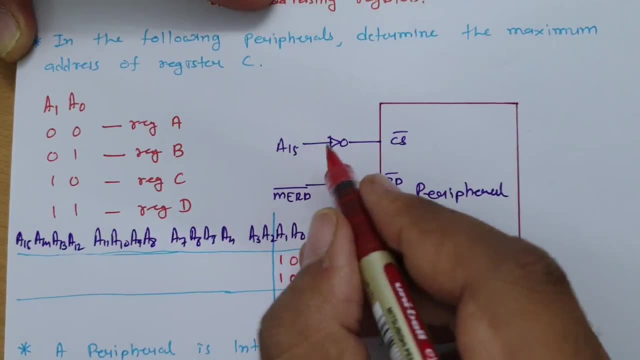 resistor C. it should be 1, 0.. Now, if you observe cheap select, that is connected with this A15. If it is 1, then over here there will be 0 and it will select this cheap. So A15, that should be 1.. 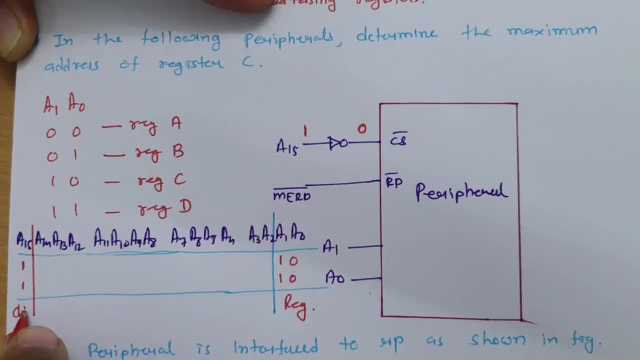 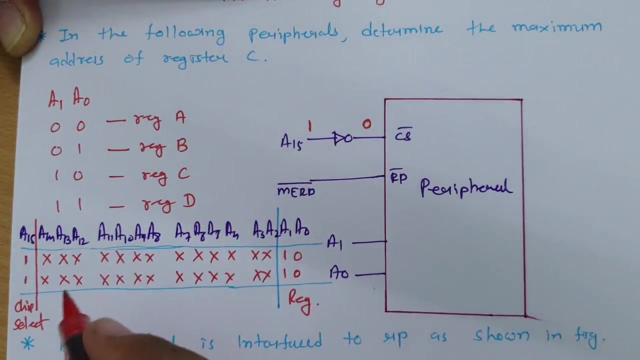 So this is what we are using it for- Cheap select- And these are don't care. The reason is we are not connecting it anywhere, So these are don't care. So question is: what is the maximum address range? So, ultimately, maximum address range that will be from 0, 0, 0 to 1, 1, 1.. 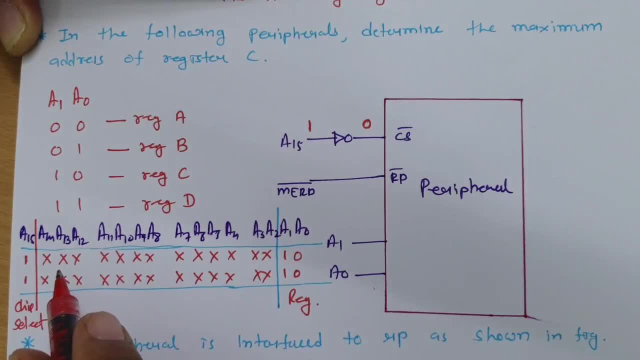 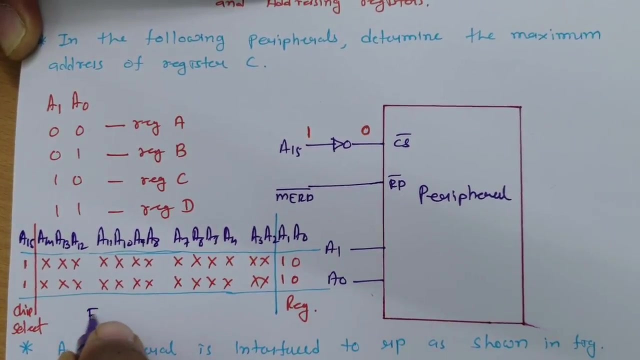 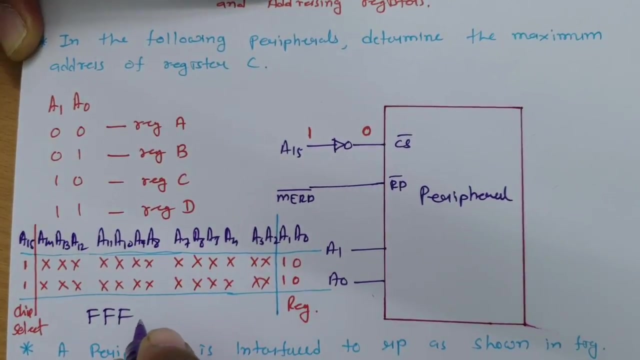 So here, if it is 0 for beginning, last will be with 1, 1, 1, 1,, right, And we can say maximum is 0. If all 1s are there, then it will be F. This all 1s means F. This all 1s means F. This is 1, 1, 1, 0 means E. 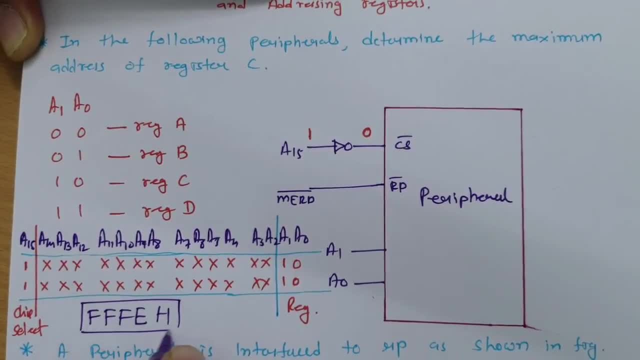 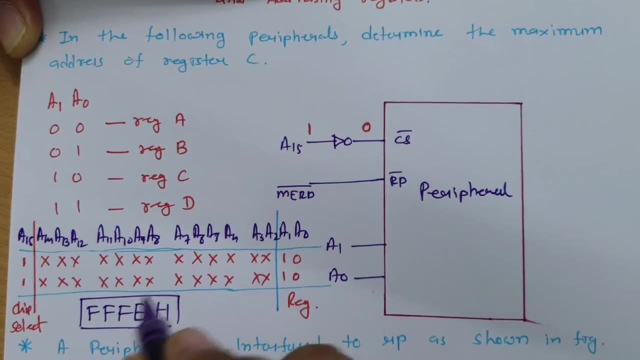 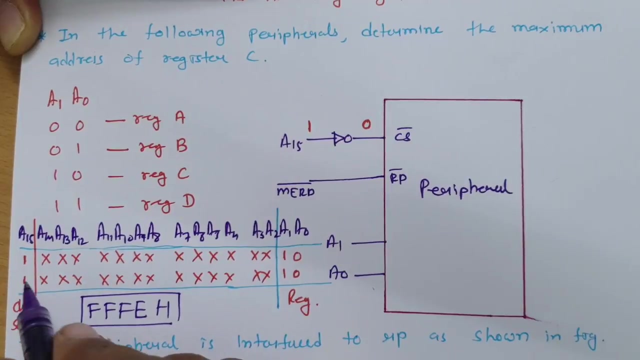 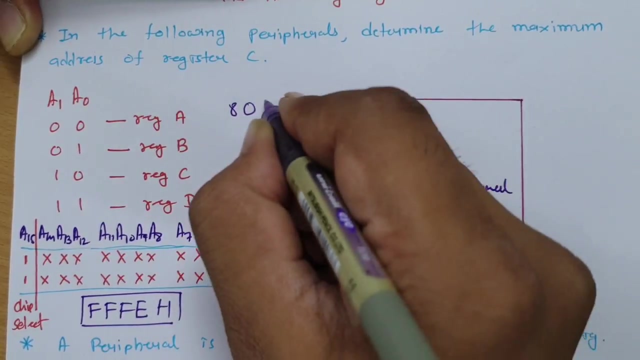 So this is maximum right. And if question is: what is the minimum, then for minimum, this don't care. That should be 0. So if minimum is there in question, in that case it should be 1, 0, 0 means 8.. All 0 means 0.. All 0 means 0.. Double 0, 1, 0 means 2.. 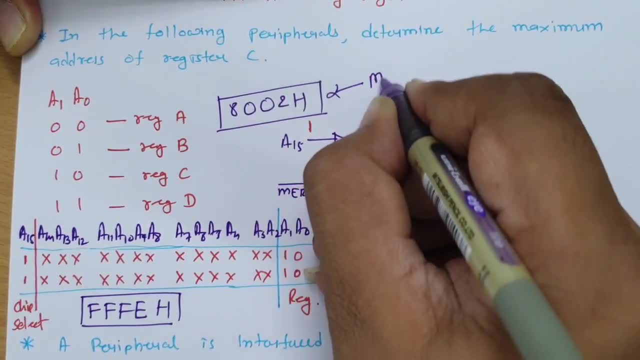 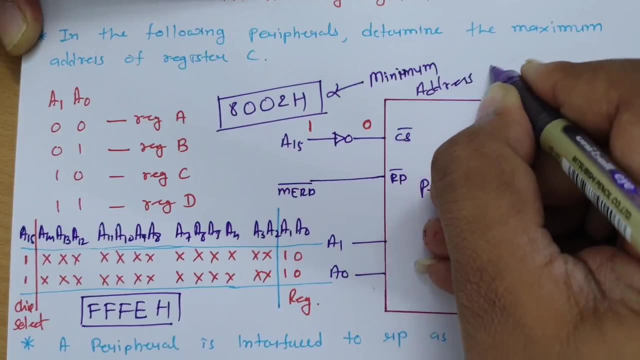 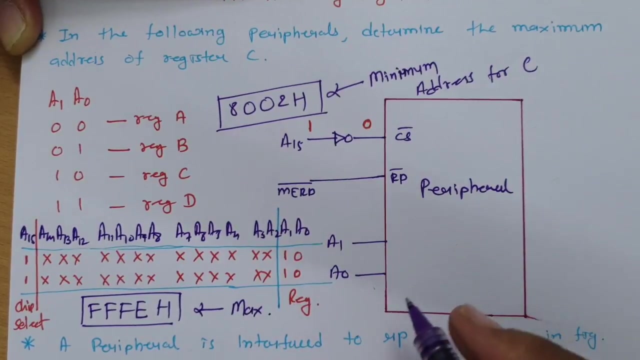 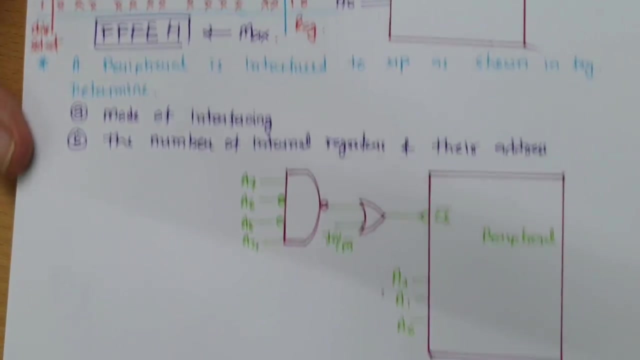 So this is minimum address. So this is minimum address for C And this is maximum address for addressing of resistor C. I hope that you have understood this. Let us have one more problem, so it will be more clear Now. see, a peripheral is interfaced to microprocessor, as shown in figure. 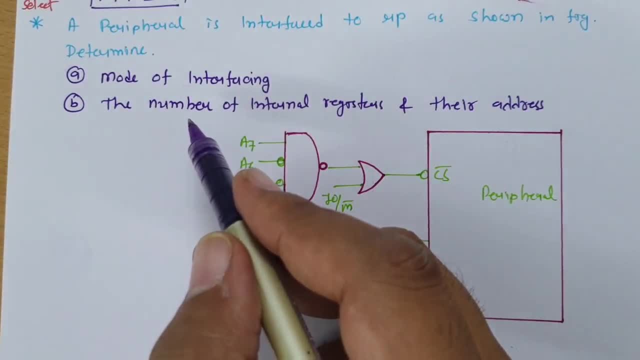 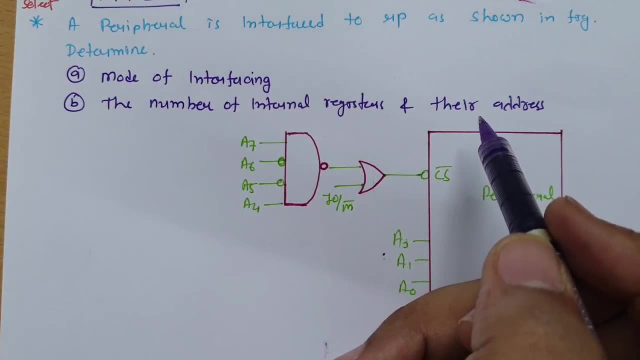 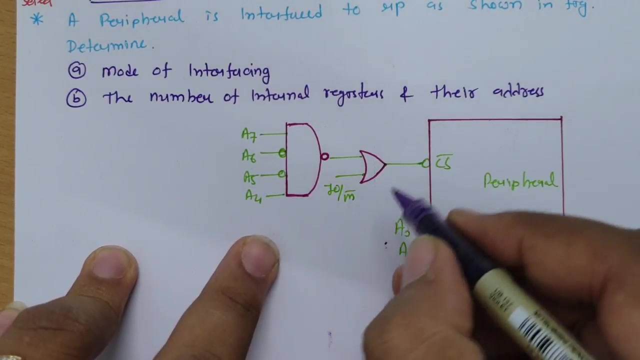 Determine mode of interfacing. And second question is: determine the number of internal resistor and their addresses. So here, if you see this peripheral interfaced C, I hope that you have understood this. Let us have one more problem, so it will be more clear. 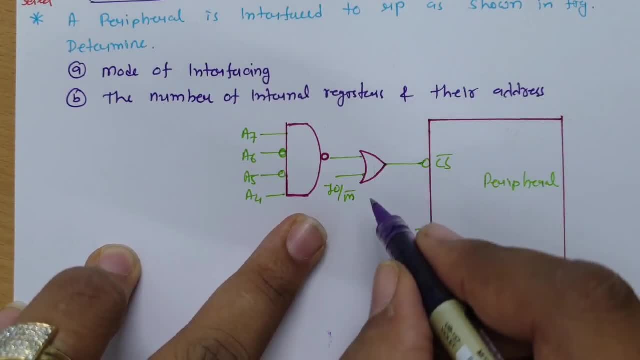 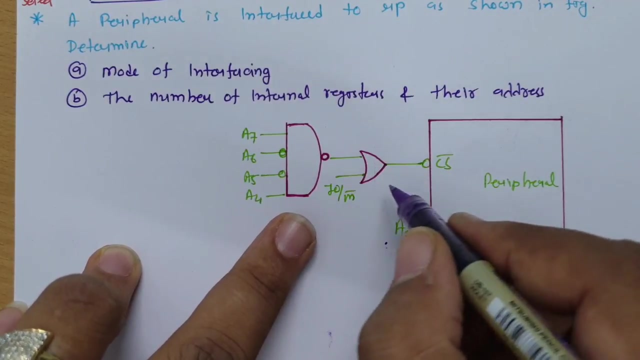 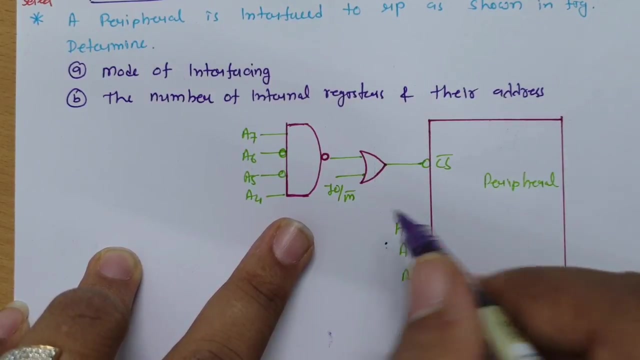 then this chip select that should be active, low, and here, if it is, if it is 1, in that case it will be addressing as io, and here, ultimately, our agenda will not get satisfied. so here, io memory bar, that is what we are connecting it here. so in io memory bar line we are connecting it for. 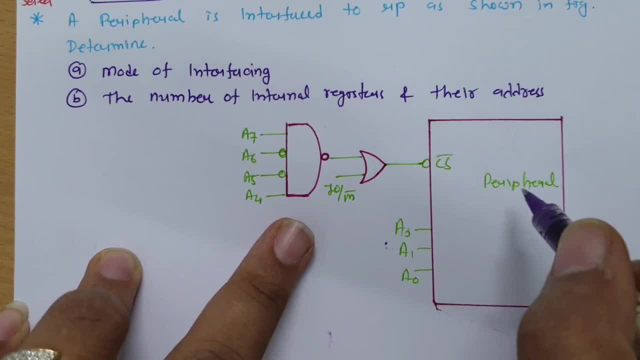 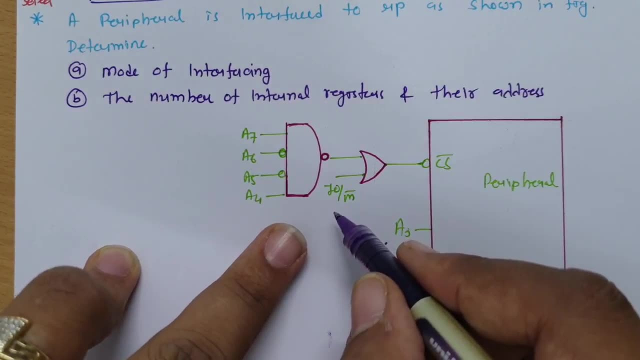 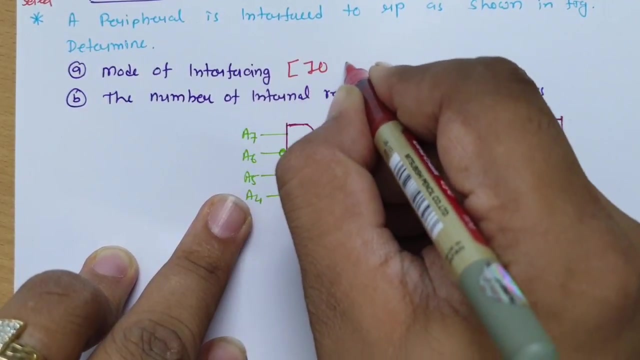 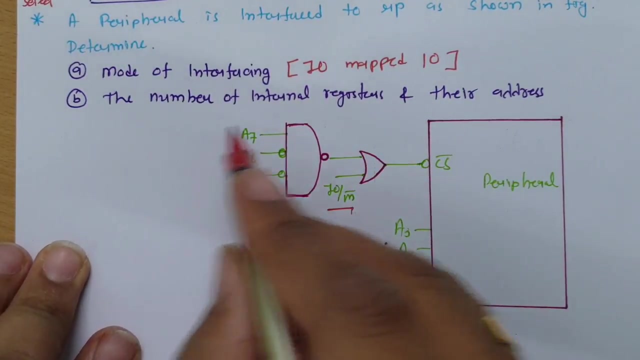 input output mapped io. so here, peripheral, that is what we are interfacing and where we are using io memory bar signal, it means this is what io mapped io. so here this line that is utilized for io mapped io. and next question is the number of internal resistor and their address. now see number of. 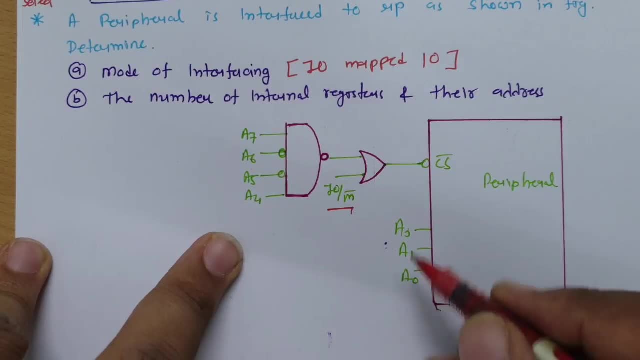 internal resistor. that is what we are having based on these three lines. so a0, a1, a3, that is what we are connecting. so a0, a1, a3. so that is having total eight selections of resistors. so if it is 0, 0, it will be selecting. 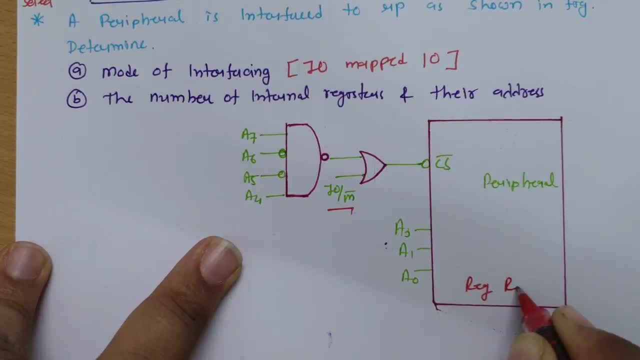 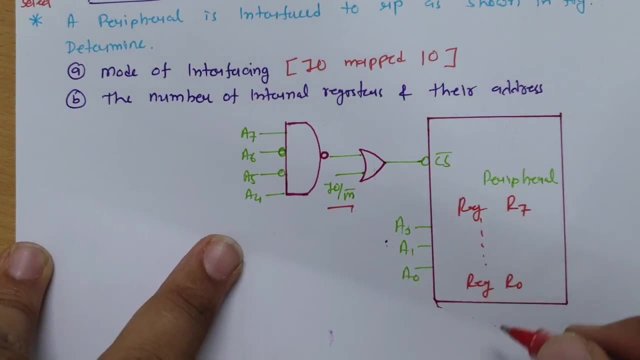 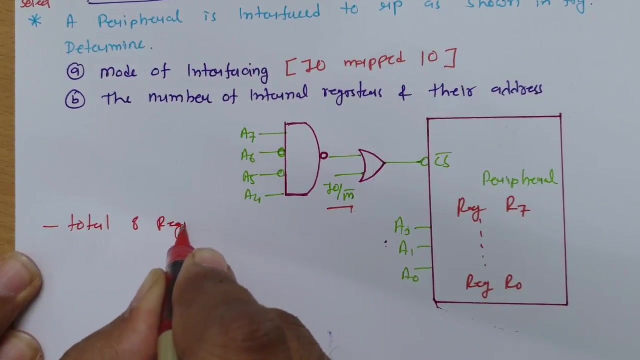 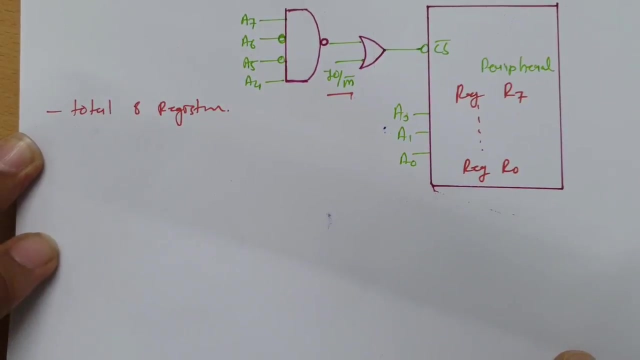 resistor 0 and if it is 1, 1, it will be selecting resistor is, that is r7. so total eight resistors are there. so total eight resistors are there. why the reason is: total three lines are there, so how we can have selection of all those resistors. so let us try to understand that. 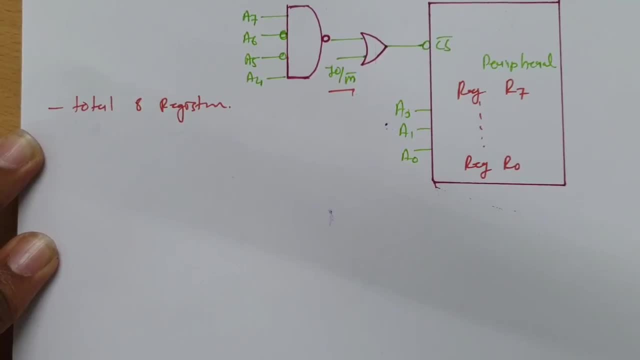 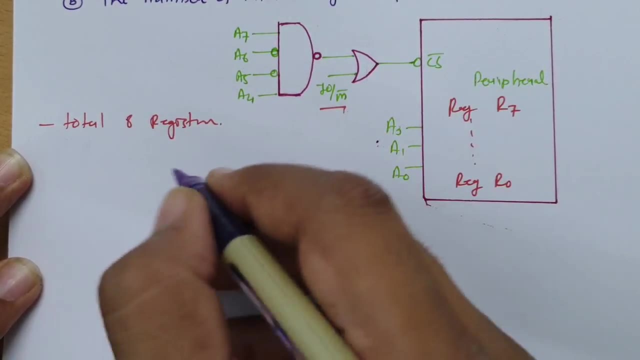 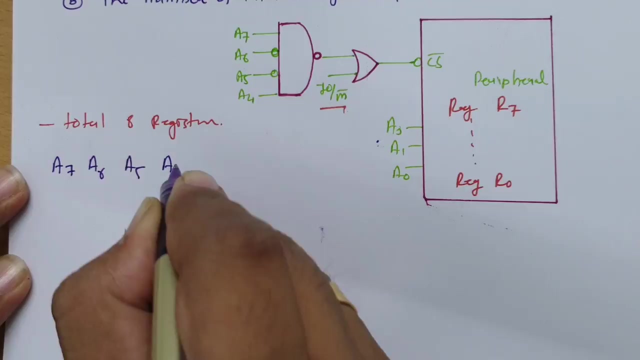 step by step. so for that, all we need to do is we need to write all address lines. so address lines are from a0 to a7, so let me mention it: a7, a6, a5, a4, a3, a2, a1 and a0. that is how address lines are there. 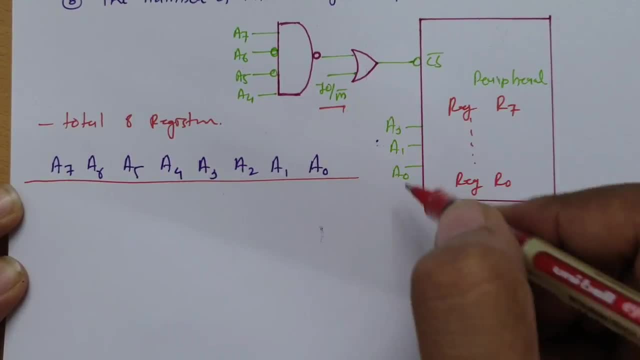 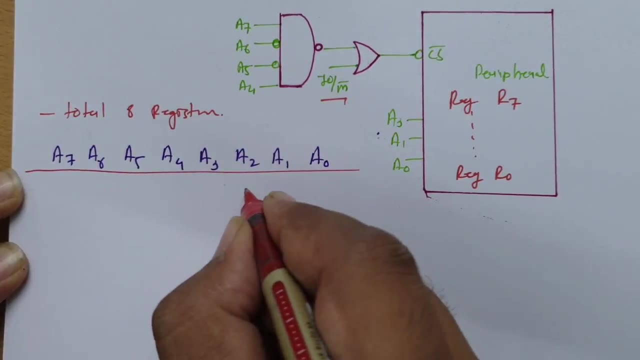 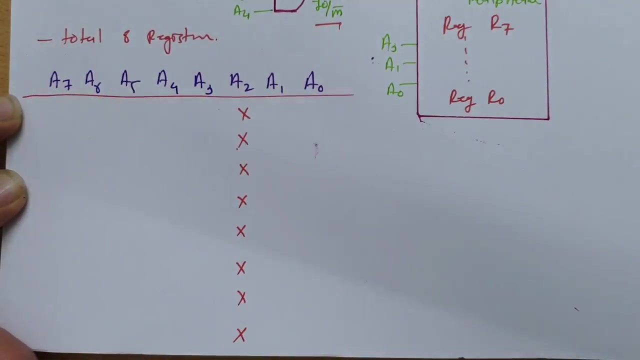 now see if you observe a0, a1, a3, a4, a5, a6 and a7, so a2, that is don't care in all conditions. so this is don't care for eight resistors. so i'll be just mentioning that it is don't care for eight resistors- 6, 7 and 8. so i have mentioned that don't care. 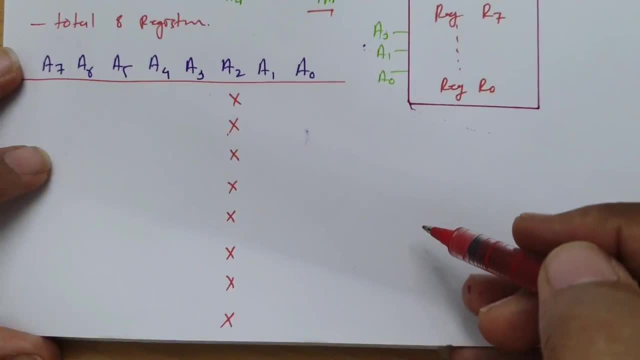 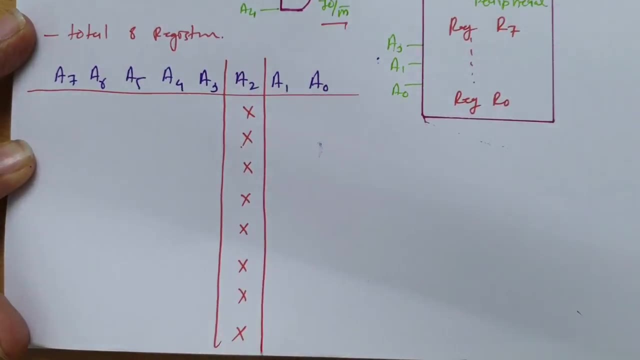 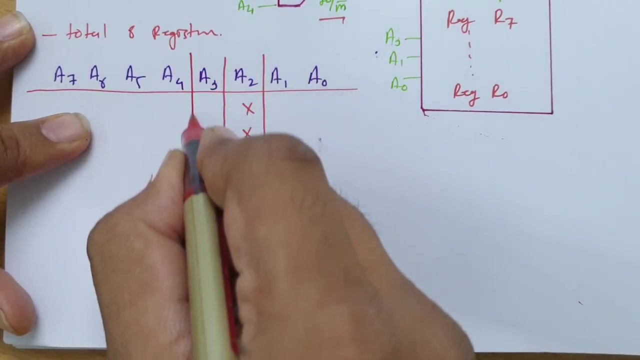 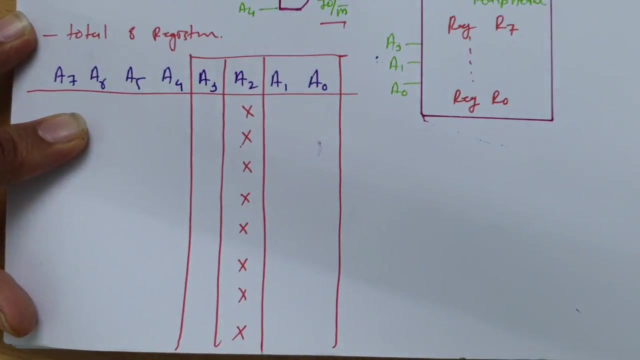 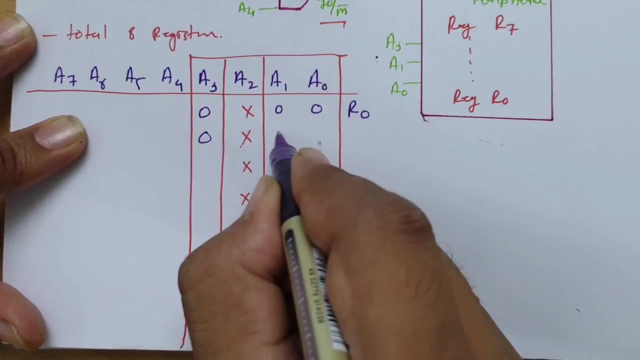 the reason is it is not interfaced here right, so it is don't care. now, here for selection of resistors, a0, a1, a3 is there. so you will be using a 0, a1 and a3 for resistor selection. So if I say this is 0 0- 0, it will be selecting register 0,. if it is 0 0- 1, it will be selecting. 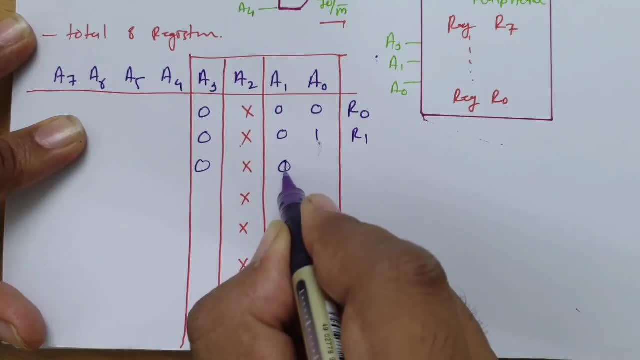 register 1, 0 0, sorry, 0 1 0,. it will be selecting register 2, 0 1 1, R 3, 1 0 0, R 4, 1 0 1,. 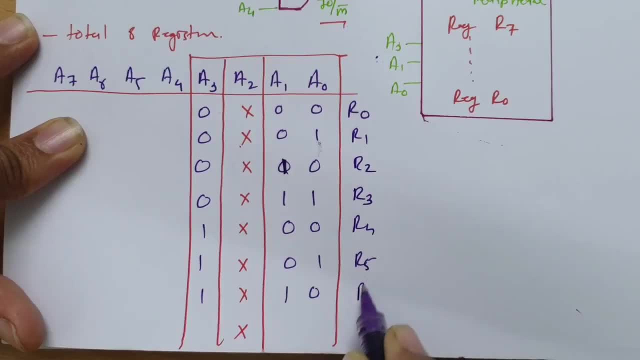 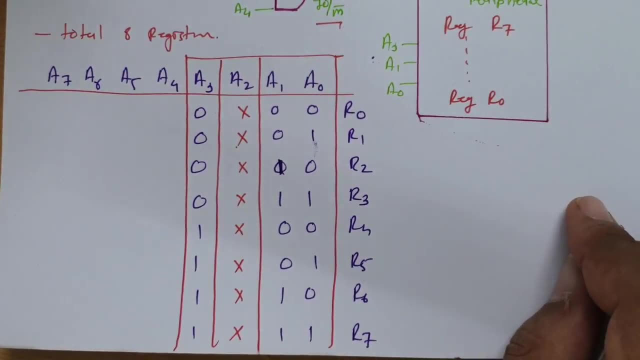 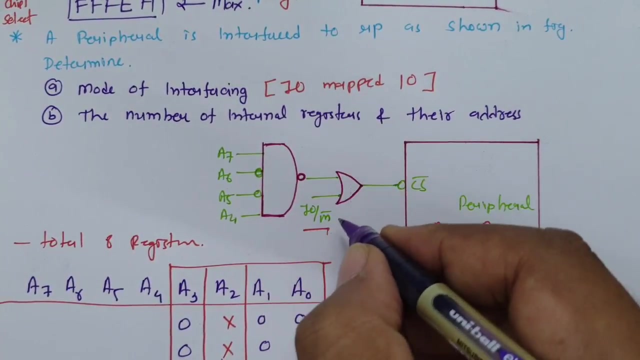 R 5, 1 1 0, R 6 and 1 1 1, means R 7 will get selected. Now this A 4, A 5, A 6 and A 7. That is what we are connecting it with: cheap select and for cheap select. this should be. 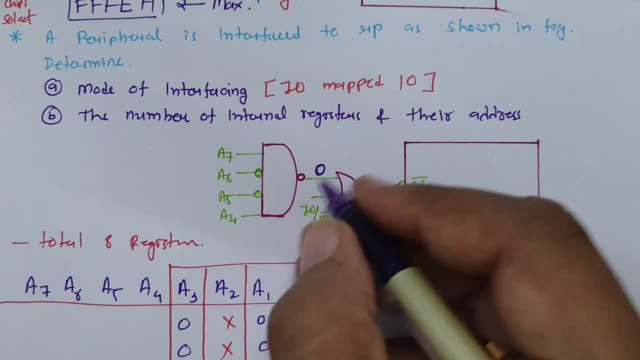 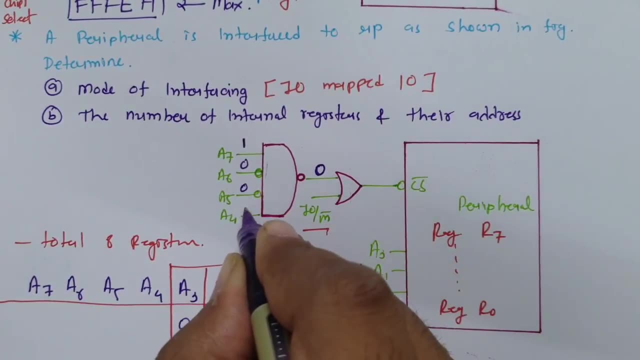 active low signal and as it is active low signal, this should be 1 for this NAND gate, this should be 0,, this should be 0 and this should be 1.. So 1, 0, 0, 1, that should be there for cheap select. 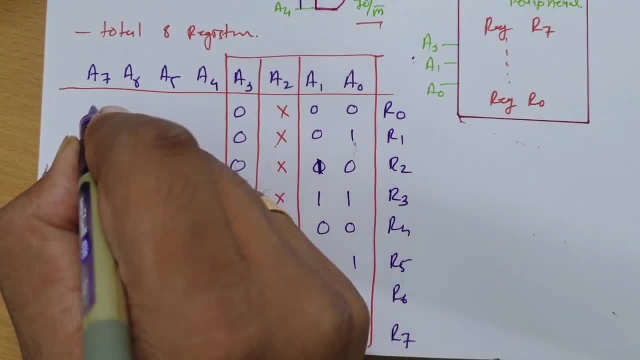 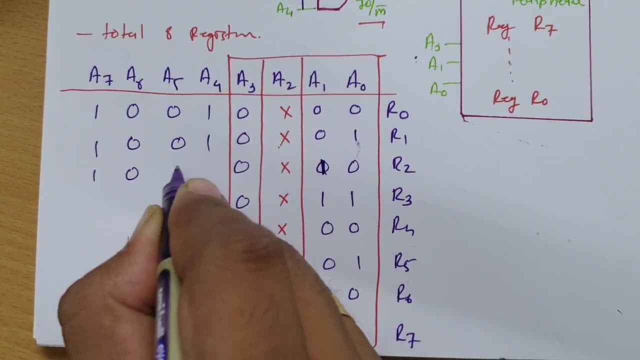 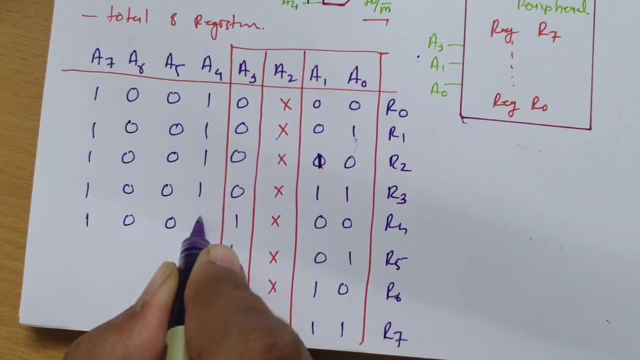 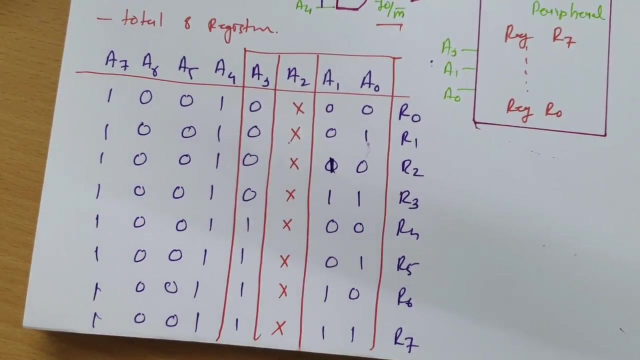 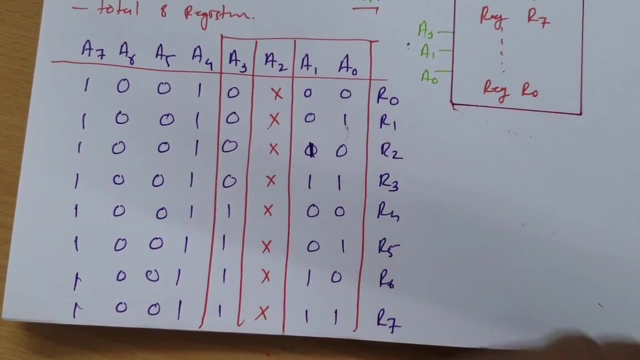 So here this data that should be 1 0, 0, 1. For all resistors. So that is how different resistors that is getting selected. Now see here: A, 2 is don't care. So there could be two possibilities that we can have. 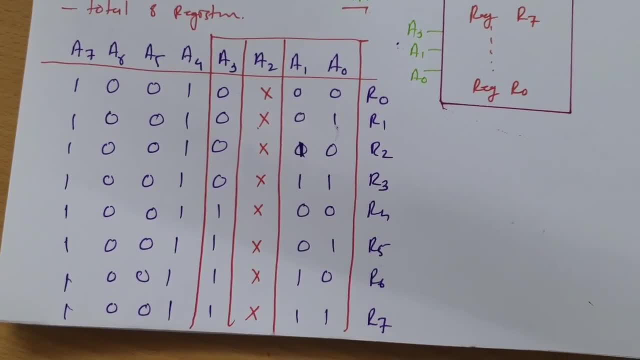 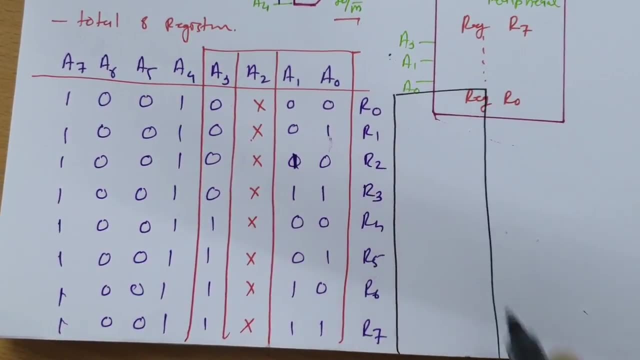 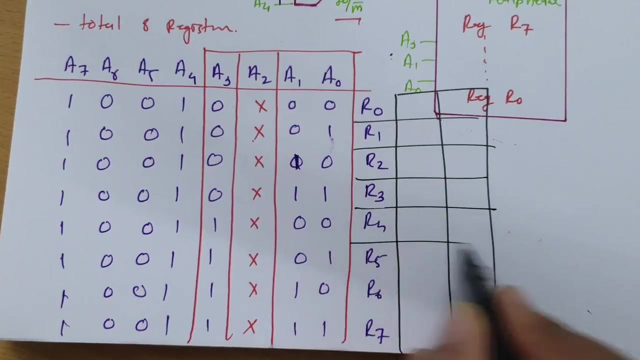 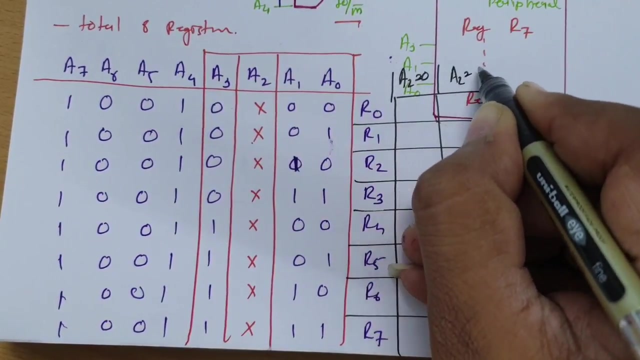 And that may result into different situations. So like see, if I say A 2. I will be writing that over here. So if A 2. If A 2, that is 0, and if A 2, that is 1.. 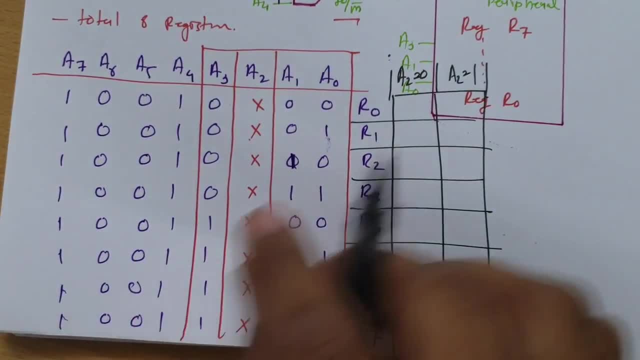 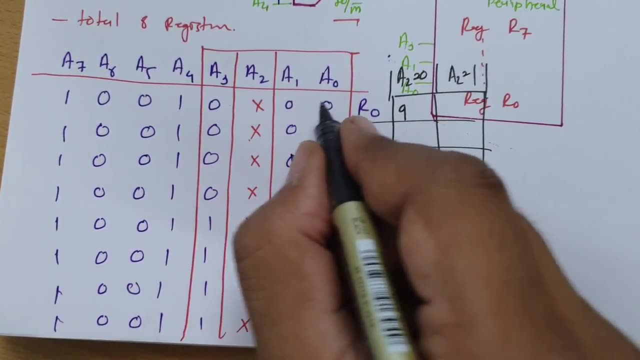 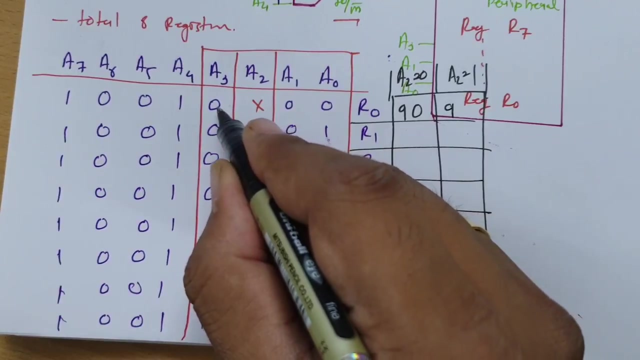 So what will be addresses? So see, if A 2 is 0.. 1 0 0, 1 means 9, then 0, 0, 0, 0 means 0.. If A 2, that is 1, in that case this will be 9 and this will be 0, 1 0, 0 means 4.. 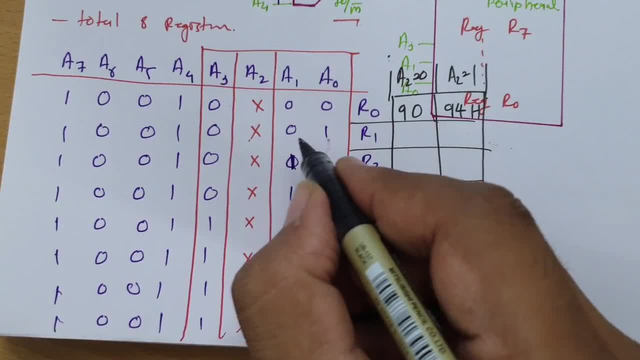 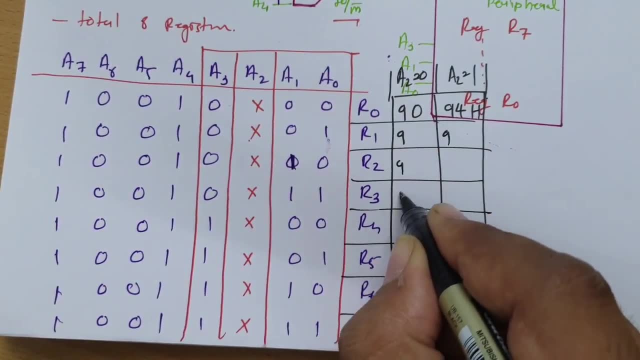 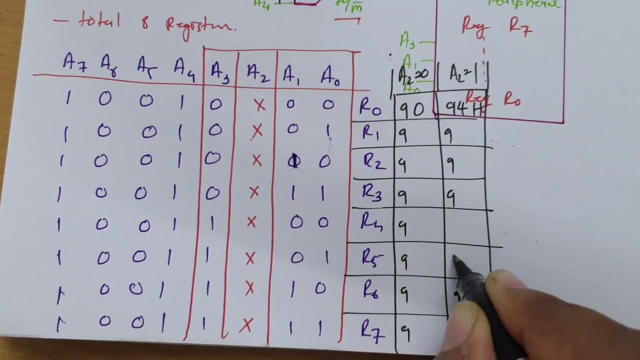 So these are the addresses of a R 0.. If A 2 is 0,, then this is 9.. See, this is 9 for all. So I'm directly writing this. Now, what about this? If it is 0, so 0, 0, 0, 0, 1 means 1.. 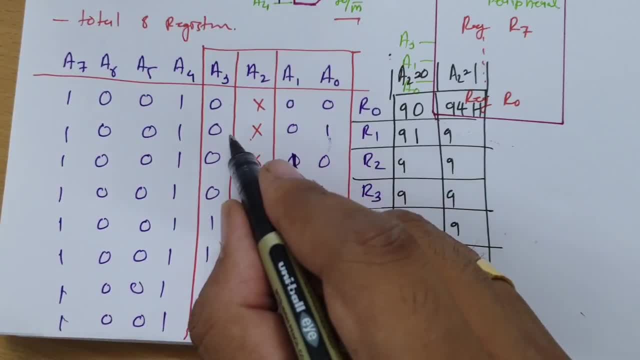 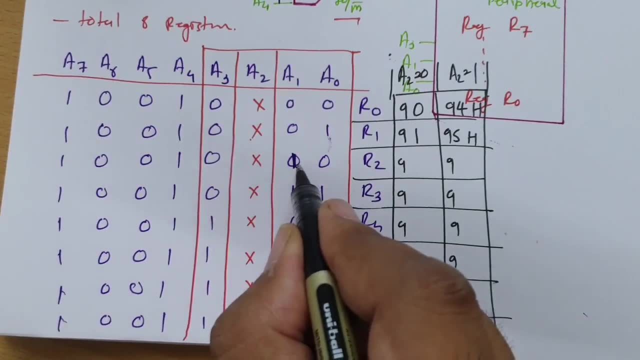 And if it is 1,, A, 2 is 1, then R 1 will be having address that is 9, 5 hex. If 0, 0, 1, 0 is there, then R 2 will be 2..